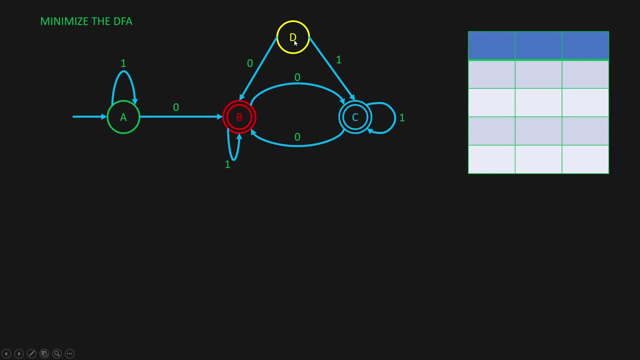 We have got B and C, which are final states, Okay. And we have got state D, But if you watch it closely, you can't reach from starting state to state D in any way. Okay, So let's say we go from. let's use the pen, Okay, Yeah. So let's say we go from state A to B. we can't reach to state. 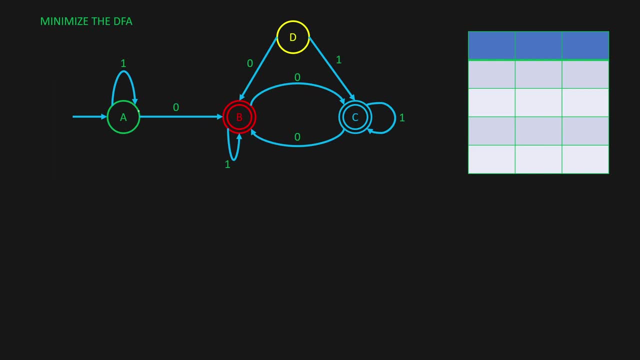 D. If you go from A to B, B to C, we can't reach to D. We can't directly go from state A to B And there is no other way to reach state D. That's why, if you can't reach state D, we will. 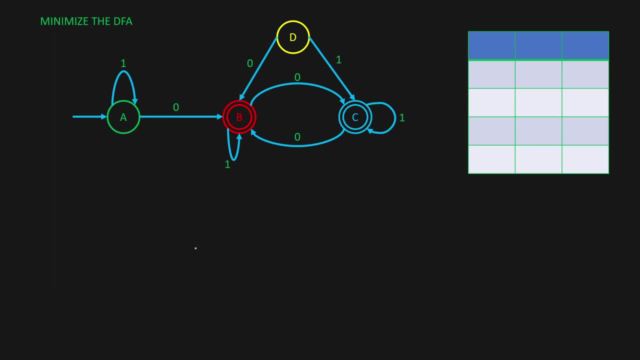 just eliminate this state, Okay. So if we eliminate this state, we'll get a new DFA that is going to look somewhat like this: We have got starting state A- Okay, You get input one. you are in state A. You get input zero, you go to state B And since state B is final, it is double circle. 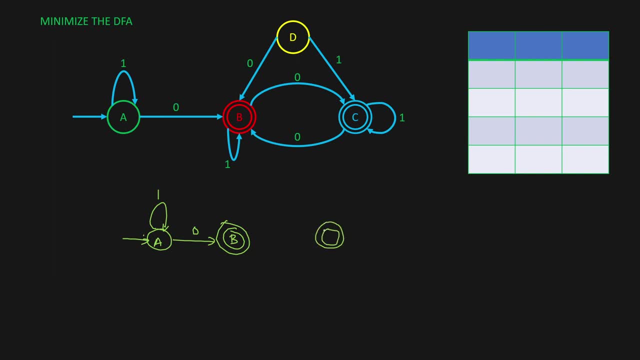 All right, Then we have got state C. over here Again, double circle. And in state B. if you get zero, you go to state C, And in state B. if you get one, you are in state B itself And in state C. if you get one, you stay in state C, And you get zero, you go to. 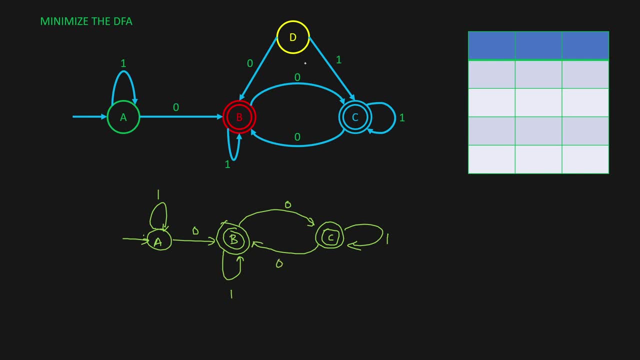 state B. All right, So this is our new DFA. Any arrows or any connection related to D state D: we are going to remove them. And we are going to remove state D because it is not reachable from your starting state A. All right, Now we'll. 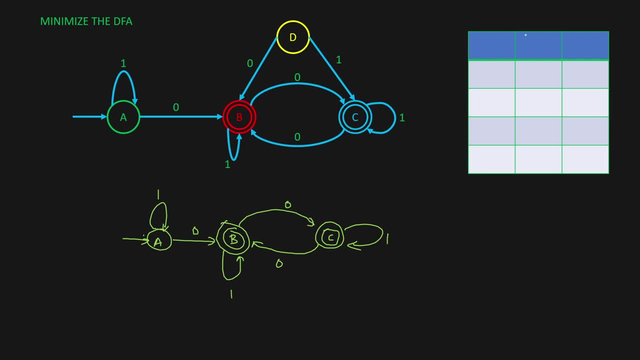 draw the DFA table, transition table for this new DFA over here. So let's say we have got starting state over here. Let's change the color. Let's say let's use color green, darker green, All right. So we have got state A over here, We have got state B and state C And inputs are zero and 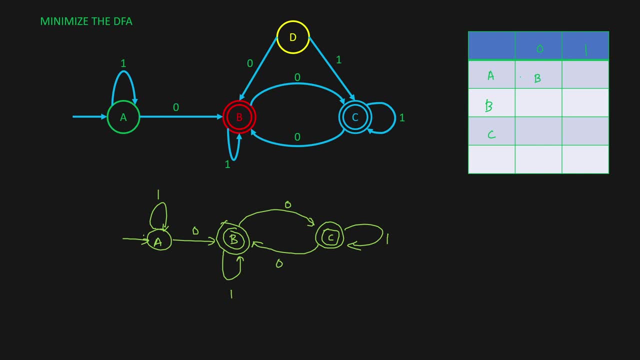 one. All right. So, on getting input zero, you go to state B over here. State A is starting state, That's why this arrow, And state B and C are final states. That's why this star mark. All right, So this is our transition table for our DFA. All right, Now the next thing that we are going to do. 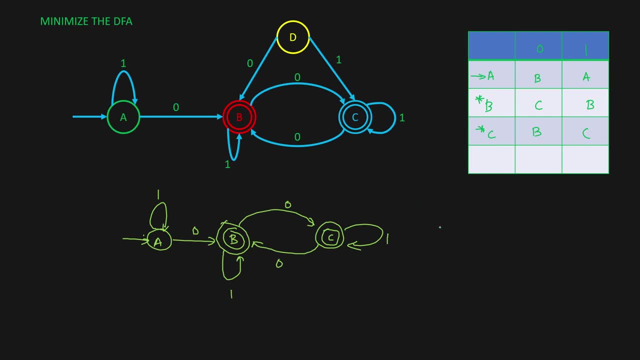 is, we are going to find equivalence of the states over here. Okay, So how do you find equivalence of the states? First thing, first, let's write zero equivalence, Zero equivalence. Now, what is zero equivalence? In zero equivalence, you divide the states into two groups: One: 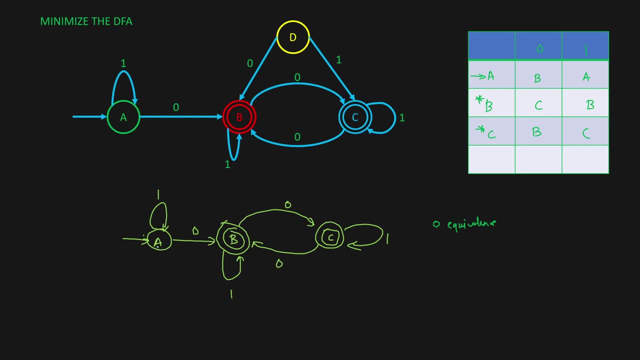 one of final states, one of non-final states. As you can see over here, A is non-final, B and C are final states, So let's divide them into two groups: A in one group and B comma C in another group. All right Now, what is one equivalence? One equivalence means when you give a certain 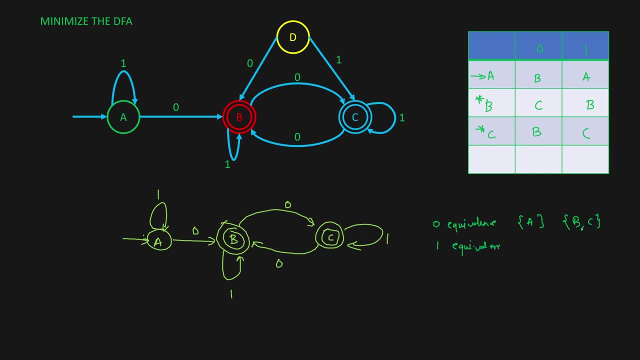 input. is the output reached from both these states part of the same set or not? Okay So let's look at an example. Let's as state A. there is nothing to compare it with. We'll check equivalence of B and C. Okay So let's look at an example. Let's as state A, there is nothing to 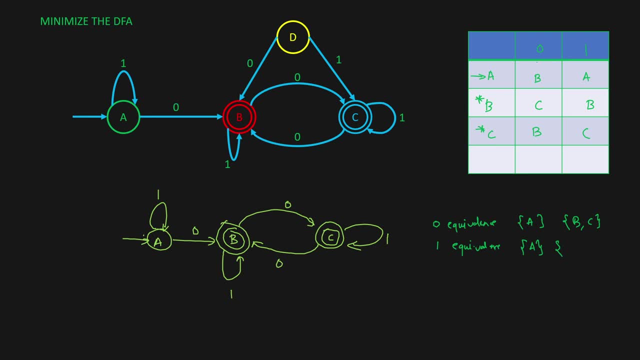 compare it with. We'll check equivalence of B and C. Okay, So let's look at an example. Let's say you are in state B, Okay, You get input zero. You go to state C. Is state C part of this set? 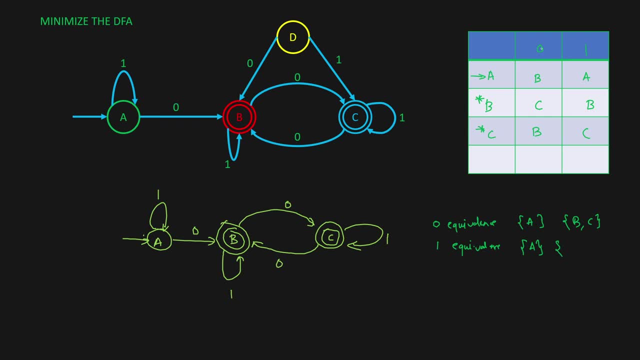 Yes, it is. What about input state C? You get input zero. You go to state B. Is it part of this set? Yes, it is. That's why, on getting input zero, they are one equivalent. What about input one? 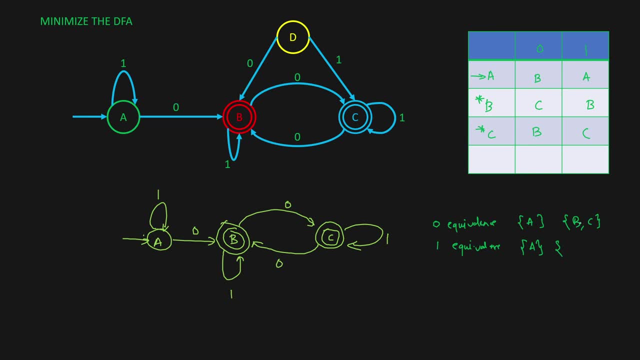 So let's say you get input one in state B, You go to state B itself. Is it part of this set? Yes, What do you? what? if you get input one in state C, You go to which set? You go to state C. 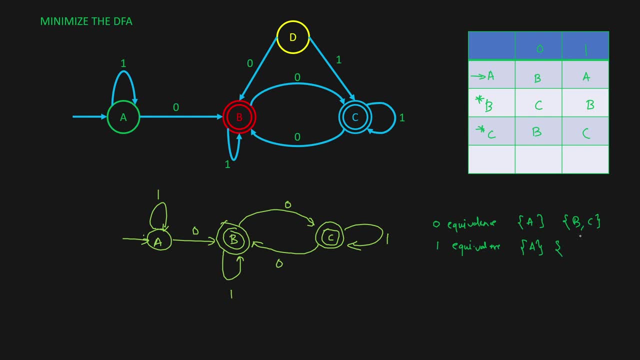 which is part of this set. So it is part of the same set of states over here. that's why b and c are one equivalent. b and c are one equivalent and since we have got two back-to-back same equivalent states, we'll stop over here. so, as we have seen, state b and c are 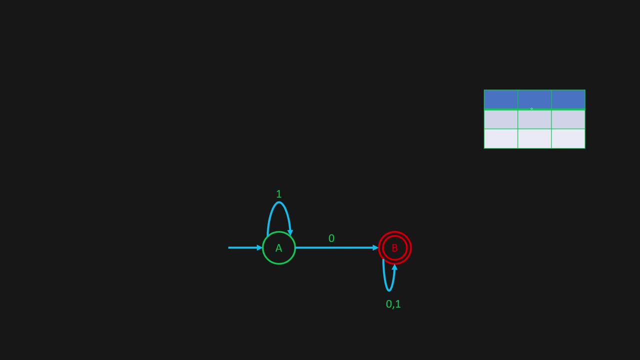 equivalent states, so we'll create a new state by combining them and we'll call it b- c. okay, so we have got input 0 and input 1 and we have got two states over here, state a and state b c. state a is the starting state and state b c is a final state. all right, so if you get input 0 in state a, 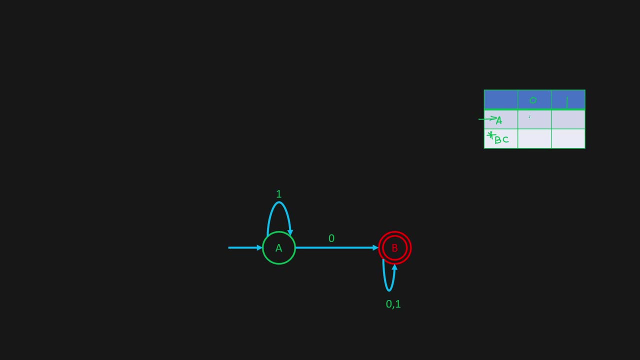 as we know, we are going to go to state b, but state b is not present. instead, we have got a new state called b c, so we'll write it as over: b c. what about input 1? you get input 1 in state a. you go to state a itself and this new state b c. what you do over here? you get input 0 or you get input.